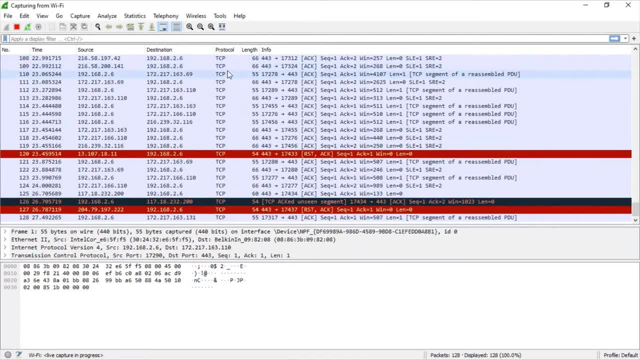 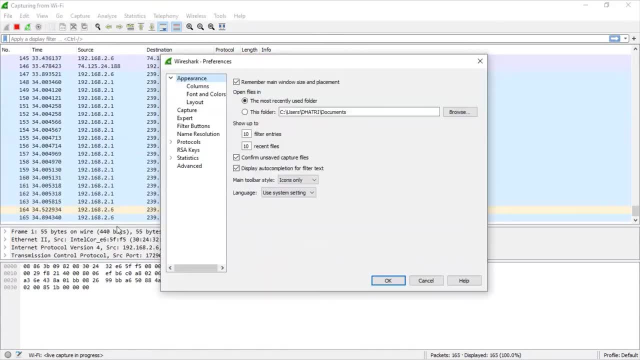 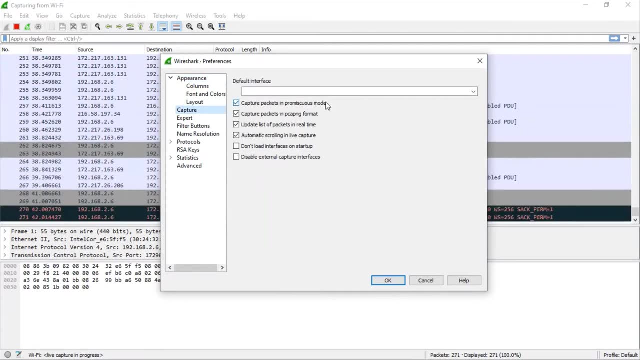 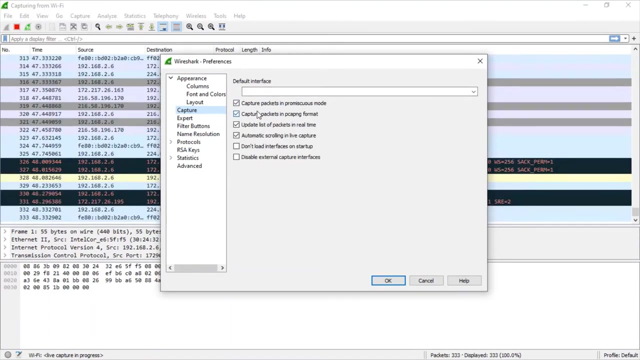 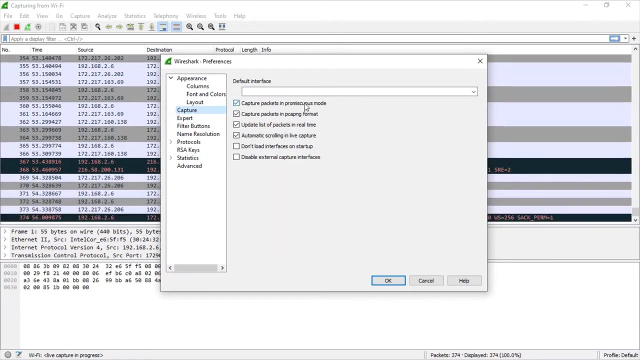 So if you want to have the network traffic in your network, you can just click on this. If you want to have the network traffic of only your device, you just have to go to edit preferences and switch off the promiscuous mode. You get that by going to the capture and capture packets in promiscuous mode. This is like you just have to uncheck the box. I want to continue doing like this, So I'm not going to do that. But if you want the traffic of only your device, you just have to uncheck the box. capture packets in promiscuous mode- It's. it's checked by default. 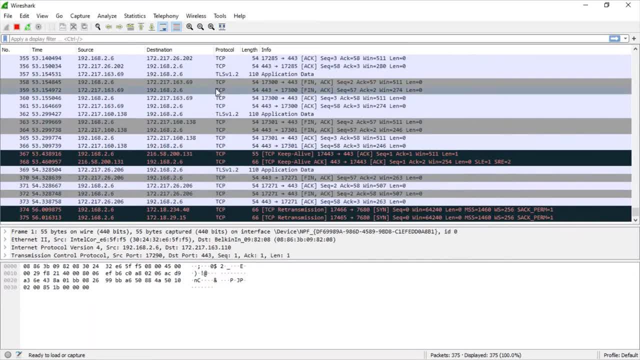 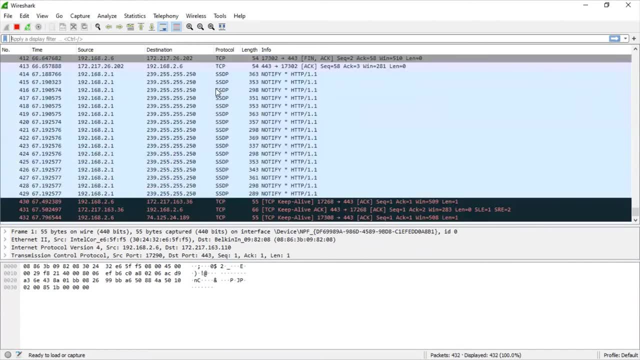 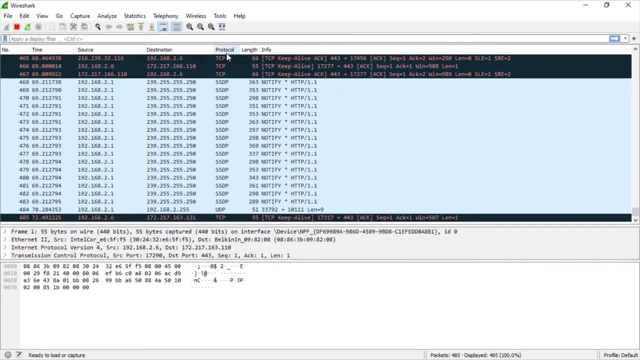 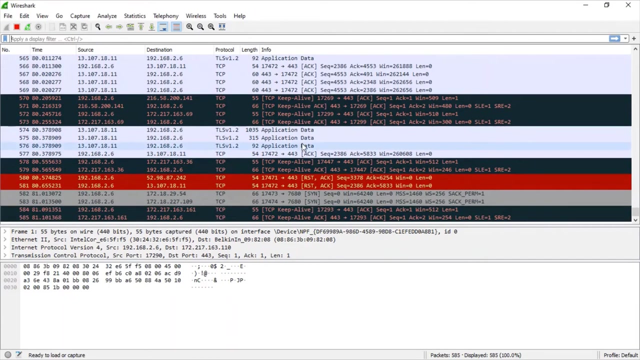 Okay and click OK, That's it. So why do we use this network traffic? You'll get to know soon. So let's start by trying something like: see you could, so now you could see all these traffic, the packets being sent and received one by one, just keeps on going like this. 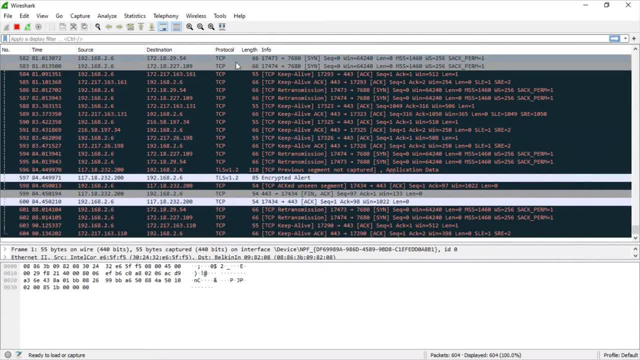 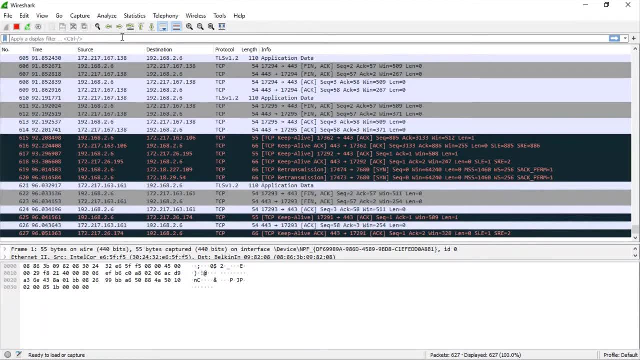 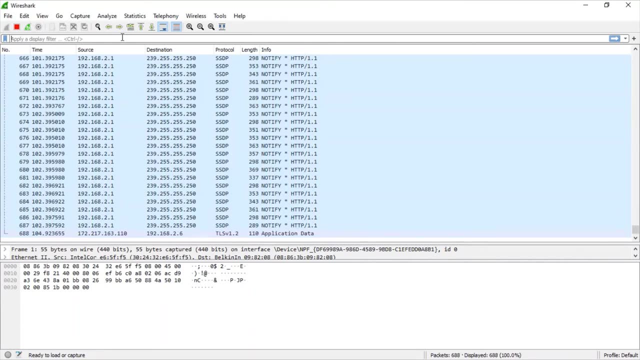 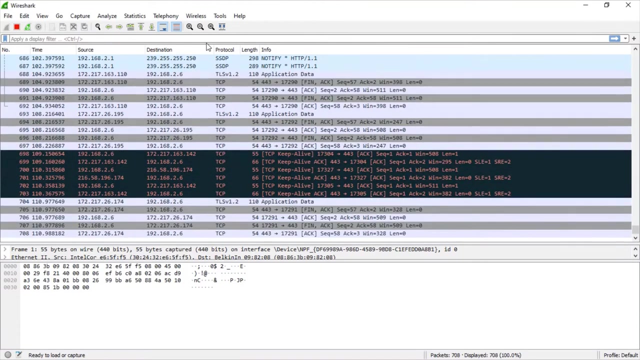 So here you could see the protocols, the TCP, the various protocols are used. So if you want to have, if you want to filter out the packets with the certain- only like specified- protocol, you want to check out it like you just have to go to this box and type the type of filter you want. like I want all the packets with the protocol, ARP address resolution protocol. So I'll just click on this. 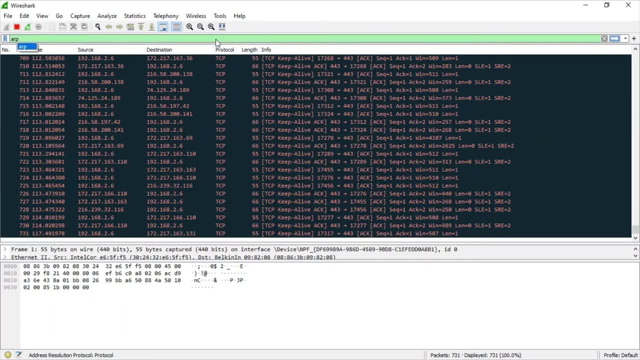 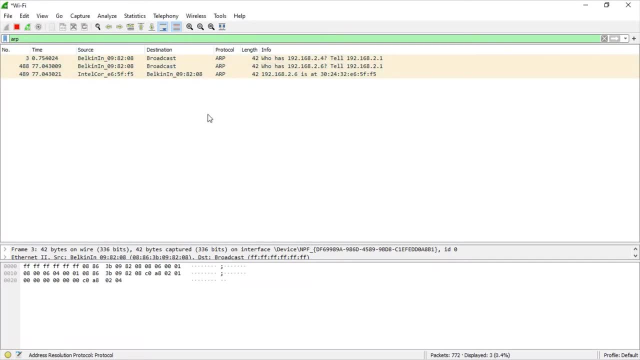 So search, I mean like input ARP, and then click enter, So I'll get all the packets with ARP in it which use the ARP protocol. So this is how it works. Before I go any further, I will be seeing about DHCP protocol and DHCP DORA process: D O R A DORA. So it's that. see DHCP DORA process. 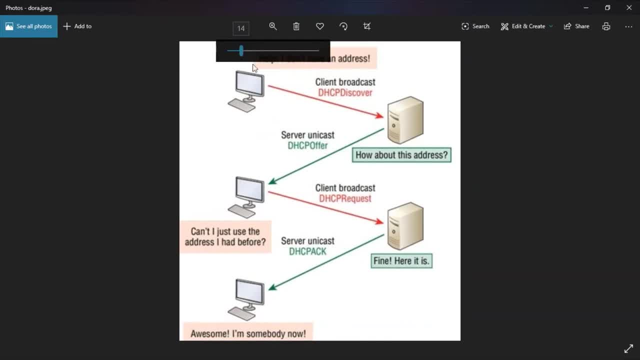 DORA is like: okay, first we need to know what DHCP is, Dynamic host configuration protocol. So this DHCP assigns IP addresses to devices or clients. So this DORA process works by first. the DORA D stands for discover, O for offer, R for request and A for acknowledgement. 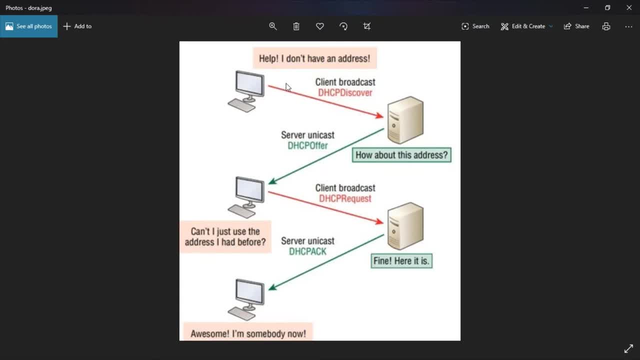 First, the client discovers The DHCP server present in the network which is it's connected to. So it just discovers the DHCP server and sends that I need an IP address, And the DHCP server responds by giving the client an offer of various IP addresses which from which it could choose from. So the client chooses an IP address and it requests the DHCP server that I want this IP address. 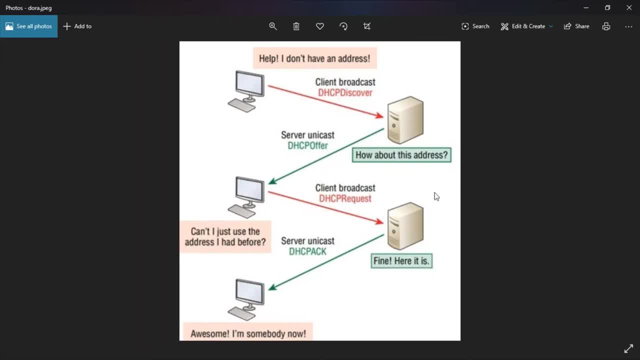 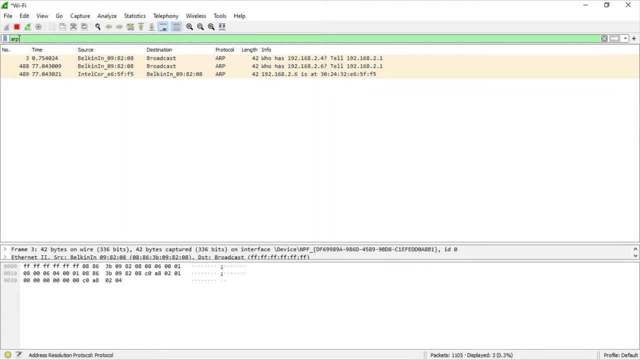 Please assign this to me. And then the DHCP then responds by saying: by acknowledging the IP address. So that's how the IP address to a client is assigned by the DHCP server. This is the DHCP DORA process. So you could go to the Wireshark and in filter you could type DHCP to know more about this. 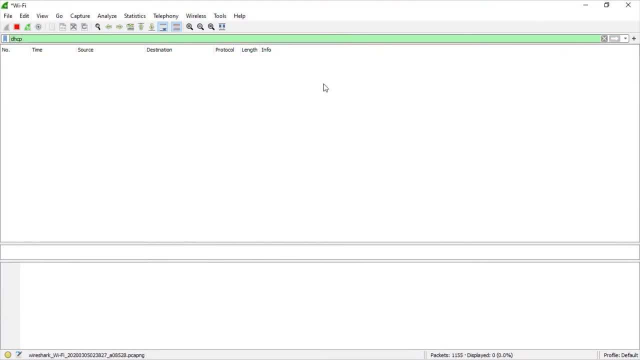 Well, currently it looks like there are no DHCP packets in the network I'm using, So there are no DHCP packets which are using the DHCP protocol. So usually if you, when you try it out, if you see that when you type the filter DHCP and when you get the DHCP packets, you could see the discover, offer request and acknowledgement process going on. 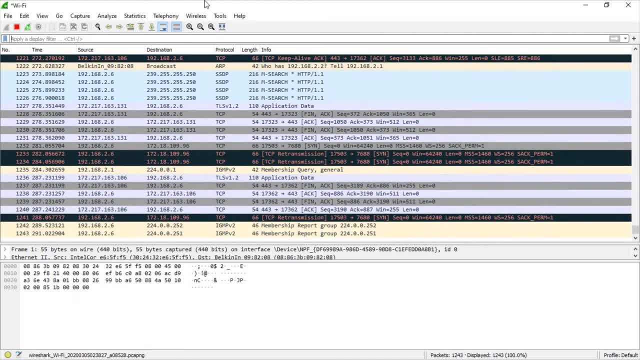 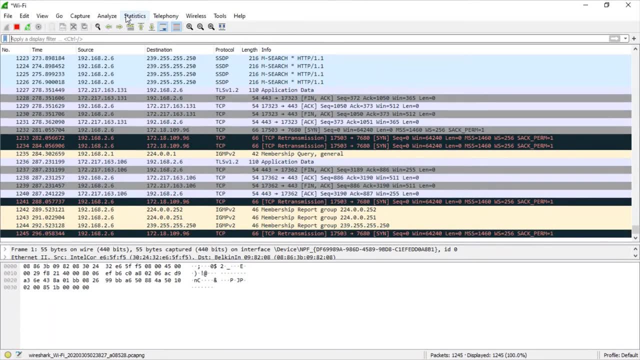 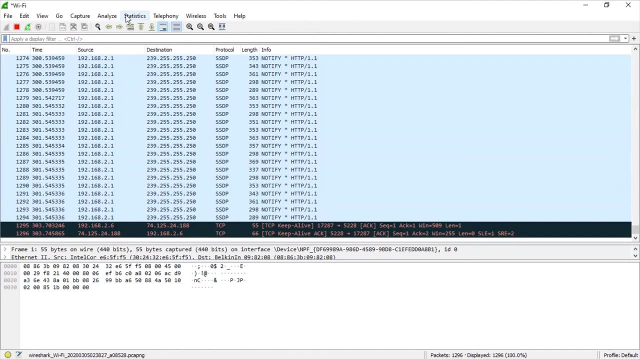 That's about the DHCP DORA process And this Wireshark. if you could see that, like I said, you could apply many filters depending upon the type, on the choice of traffic you want. So if you want it for a particular device, like a device that not the host device or the device which you're using, but a different device in your network, you just want to analyze the traffic of a different device in your network, you have to go to statistics. 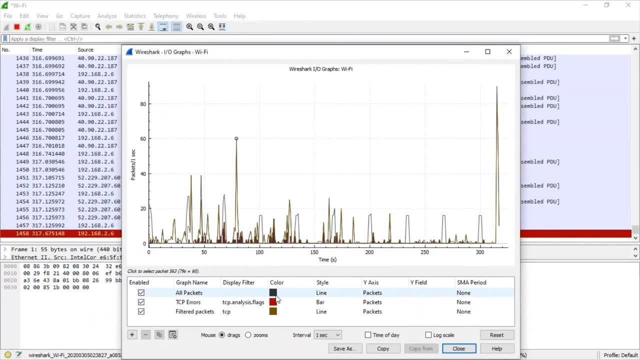 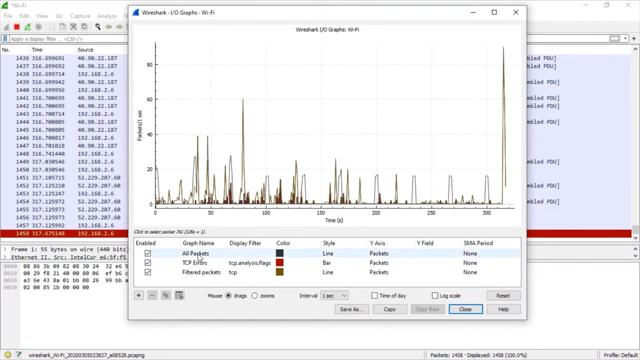 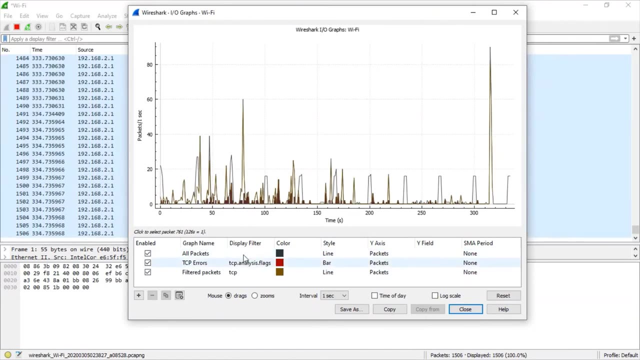 Here you could see that all packets and you could see the graph of all the various packets here And down. here you could see all packets, TCP, RS, filtered packets and all that Just go to this display filter here in display filter. All you have to do is double click here and type the IP address you want to analyze, for which you want to analyze the traffic for. 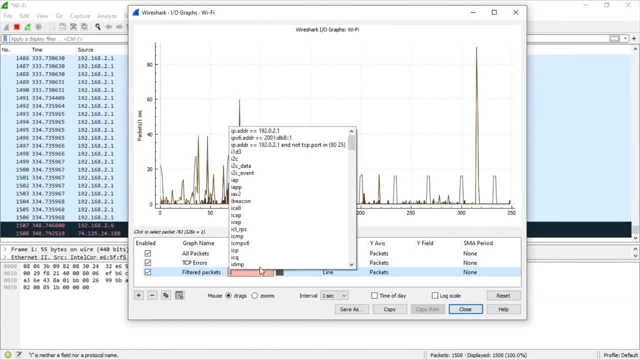 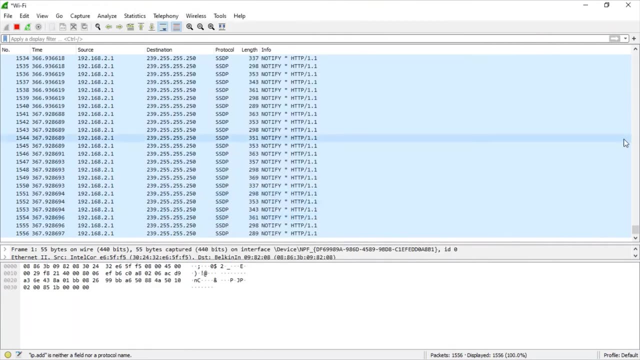 So all you have to do is type IP dot- ADDR. See, we already get it in the solution: ADDR, equal to equal to the IP address. So that's how it works Like. so when I minimize, you get the traffic only for the that particular device. you get all the packets sent and received to that device. 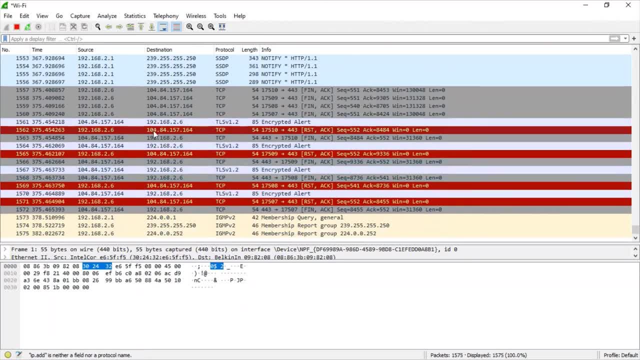 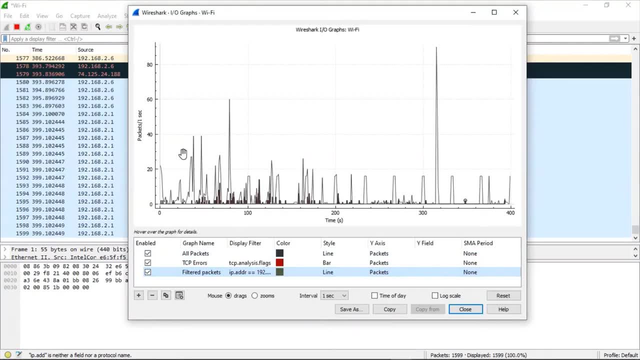 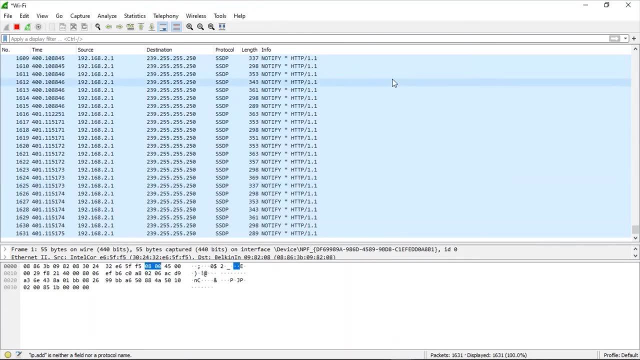 You could see. now you could see the IP, or destination IP address and source IP address are only going to be The IP address which I gave. Yeah, I gave the IP address 192.168.2.1.. So you get all that, all the traffic related to that IP address. So this is how Wireshark works, And why do you need this Wireshark? So it has many different purposes. One of it's one could be that it could actually be used as a security tool. This could be used. this Wireshark tool could actually be used to identify a DOS attack. 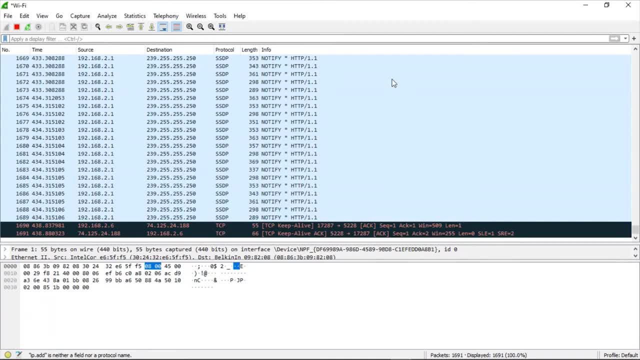 DOS or DDoS attack. DDoS or DDoS is just a denial of service- denial of service- And DDoS is distributed denial of service. This is a type of attack. This is a very common attack, where the attacker actually bombards the particular host website with multiple requests or multiple requests. 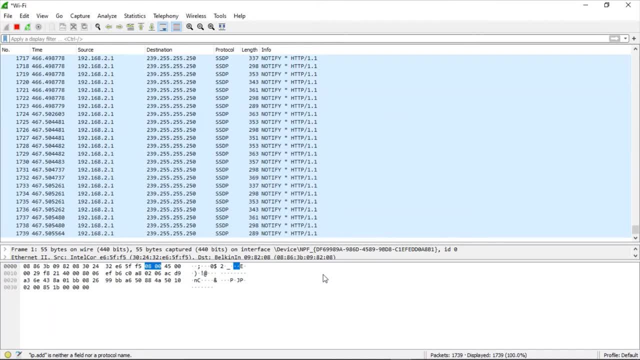 This could actually lead to Slowing down of the website or, in worst case- and I use, crashing of the website. So what the attacker does is just bombards the website with multiple requests, Many requests actually like, some more than the more requests and the website could actually handle. So that leads to the crashing of the website, And if the website is down for even a few minutes, it could actually cause a great loss to the website. So how could you? 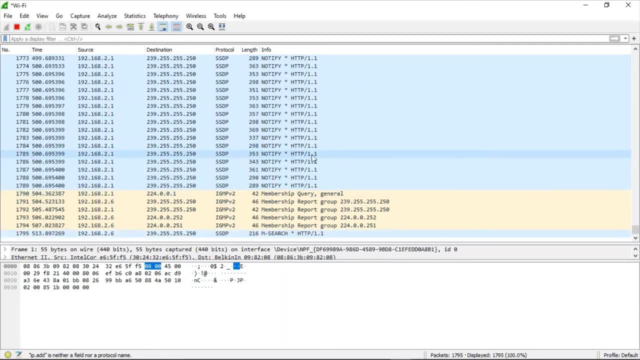 Identify the DDoS or DDoS attack is simple, It's just that you could, And just by analyzing the traffic you can understand right, It gives you multiple requests, multiple, a lot of requests, a lot of. you start receiving a lot of packets from that source IP address, So from the source, So you could easily tell that this is a DDoS attack or not. But sadly Wireshark could only just identify the DDoS attack.